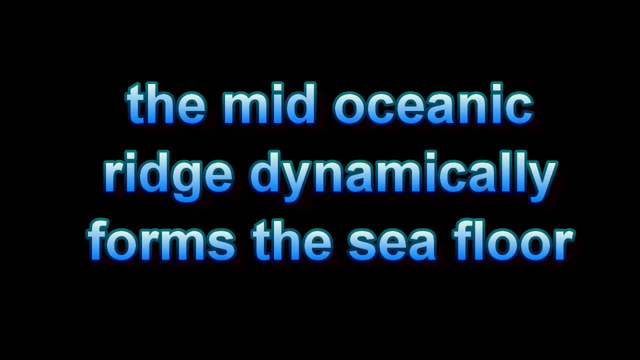 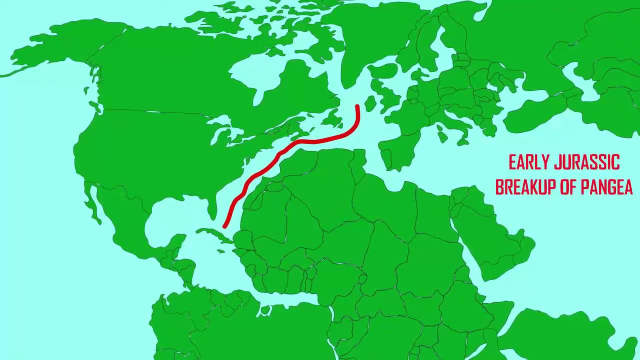 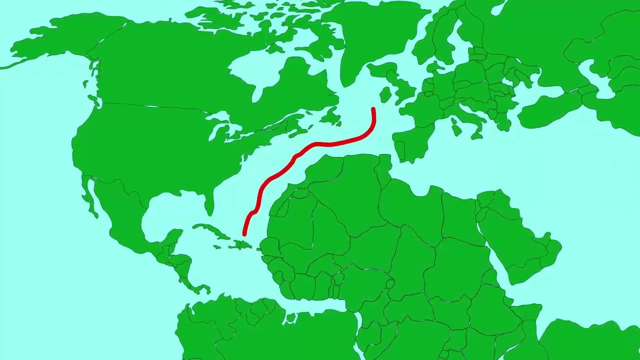 The magnometer readings indicated that the ocean floor is not the stable structure, but rather it is continually formed, at mid-ocean ridges, For example. the mid-Atlantic ridge, then, apparently, is where the floor of the Atlantic Ocean was formed, It seems the continents. 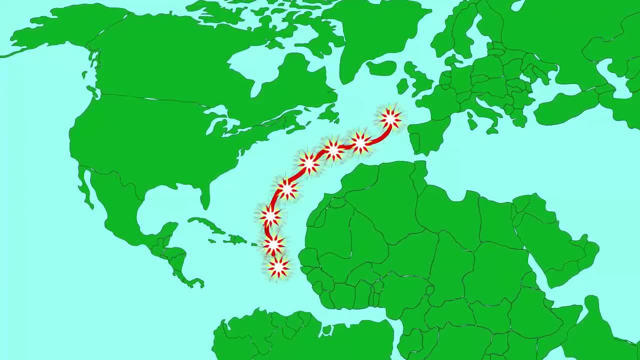 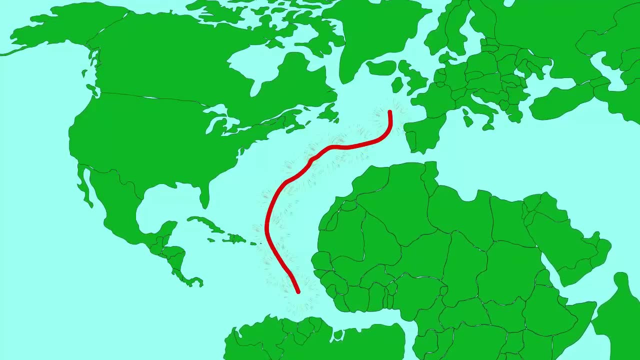 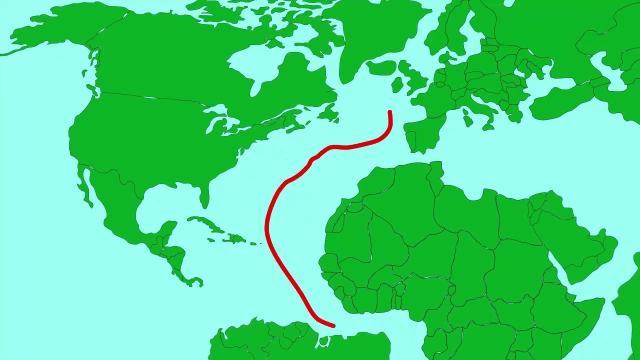 once formed a supercontinent called Pangea, which then split, starting in the early Jurassic in the North Atlantic and then continuing into the South Atlantic by the Cretaceous period. So the continents were pushed apart as the mid-Atlantic ridge formed new sea floor. 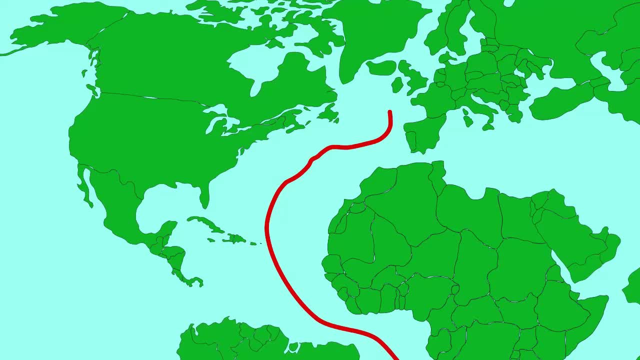 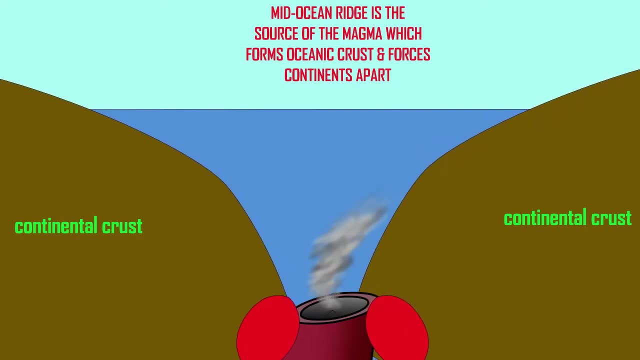 from the magma which welled up from the mantle. These readings have been confirmed With age calculations of various points on the ocean floor and are consistent with the sediment buildup over the ocean floor, which is thinnest at the mid-ocean ridges and thickest 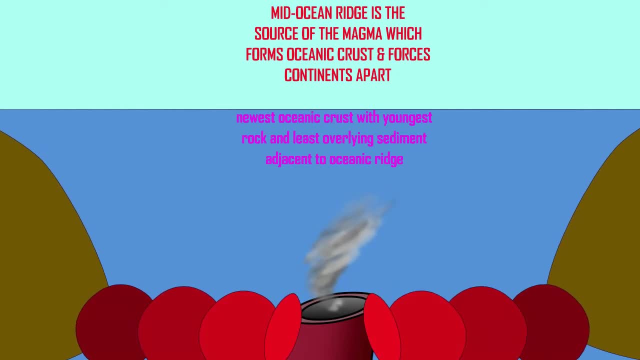 near the continents. It appears that the mid-ocean ridges are the sources of the magma which then solidifies and forms new ocean crust Over time, and in this animation the older crust is depicted by the darker shade of red. the addition of 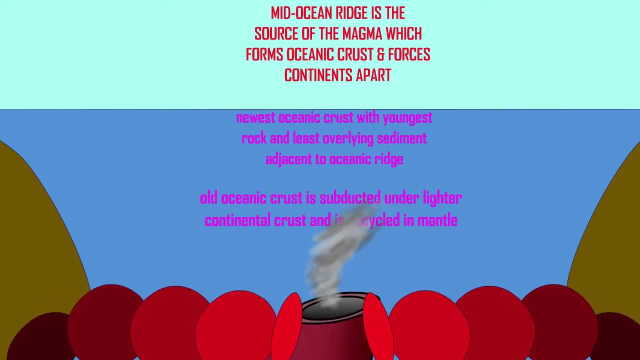 new ocean crust forces the continents farther apart, and the ocean grows. Ocean crust is not permanent and at some point this denser crust then is subducted under the lighter continental crust. Once this is directed towards the mantle, it will then become magma once again and can be recycled eventually. 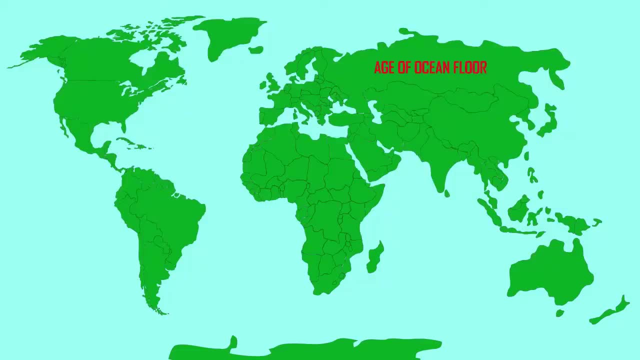 forming new ocean crust, Thus throughout the oceans of the world. the youngest crust, which dates to the Pleistocene to Pliocene epochs, from 0 to 5 million years ago, this crust would be found along the mid-ocean ridges.